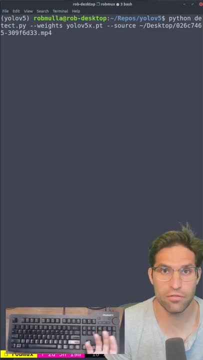 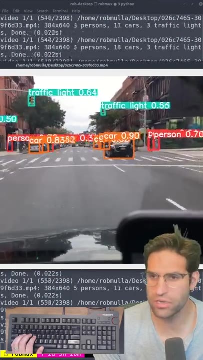 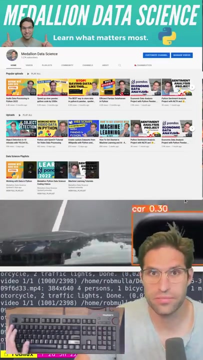 own data set. You don't have to use your webcam. you can run it on a video file. Just add view image to see the image as it detects. This footage of a car driving shows all the detected objects. Subscribe to my channel to see a longer youtube tutorial on running object detection. 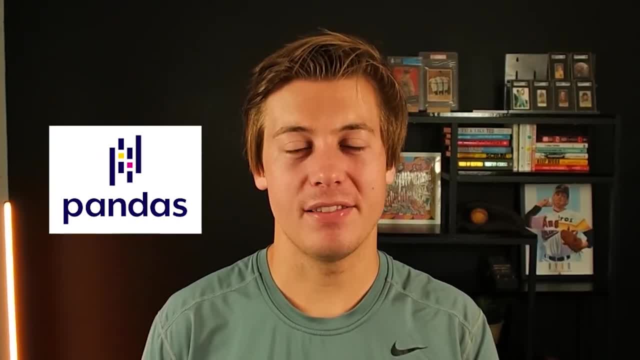 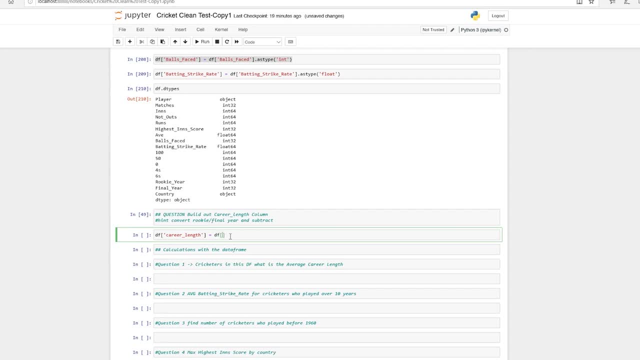 Today we're going to be taking a look at how you can clean up data within pandas. In fact, we're going to be dropping both rows and columns. We're also going to be creating brand new columns or series. is manipulating some strings, changing data types as well as debugging an issue Now. 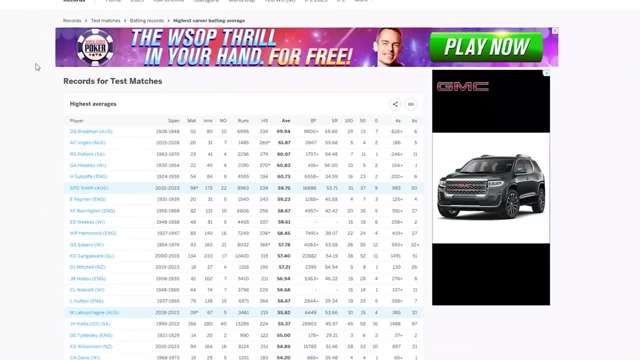 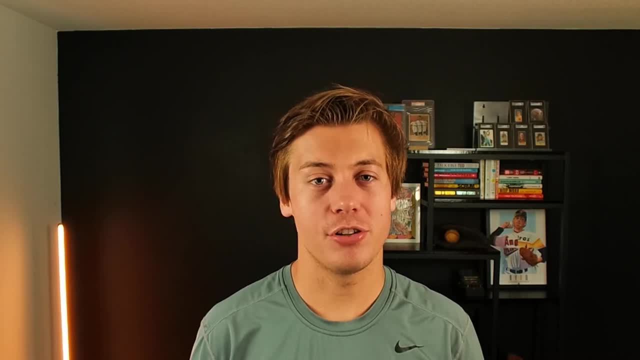 the data we're going to be using today is pulled directly from ESPN. I'll should be showing you how to import that, And we're going to be taking a look specifically at some of the best cricket players with the highest batting averages in test matches And, with that in mind, I'm going to jump. 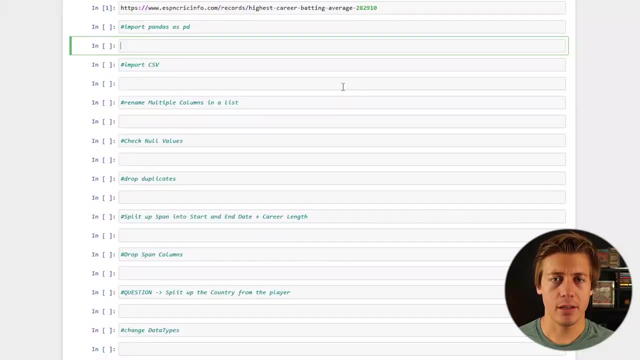 on my computer right now and let's start cleaning up some cricket data. So before we can clean up a spreadsheet, I have to grab the data. Now I'm grabbing info from ESPN cricket infocom, So I'll show you guys what we can do. So I'm just going to open up a new tab over here and load this up. 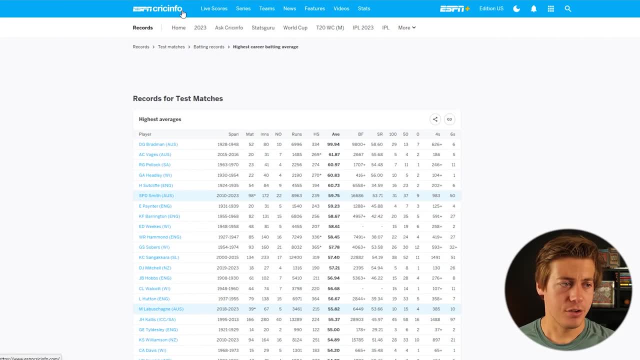 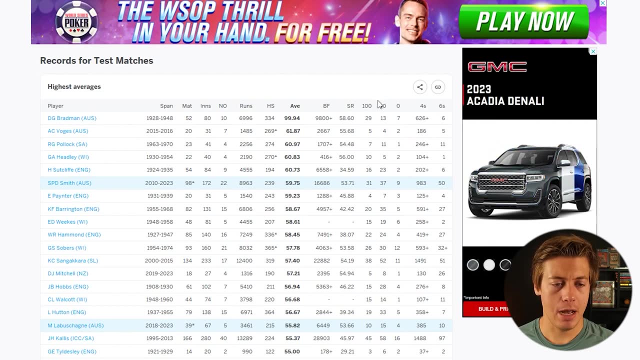 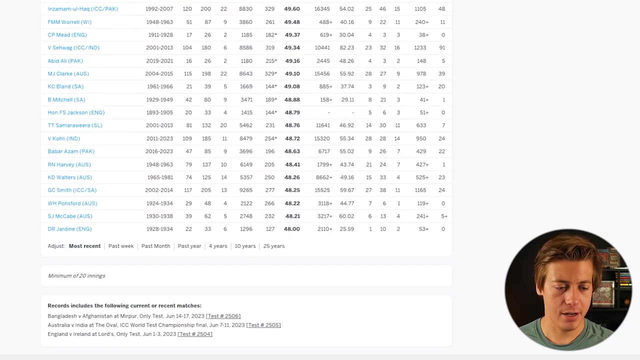 and show you what this specifically looks like. So we have this over here and this is different data from test matches. Now, I can't really grab this as a CSV. uh, some sites that have data, uh, you can, but this one does not right. There's no option.